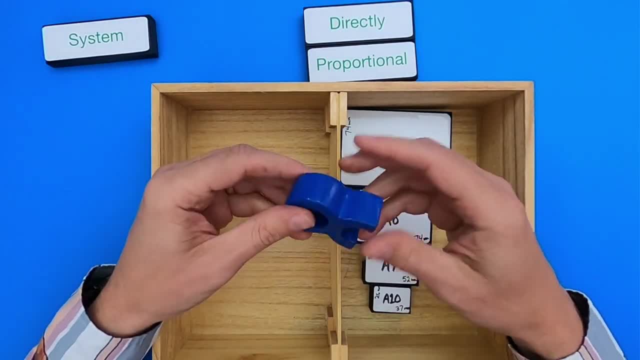 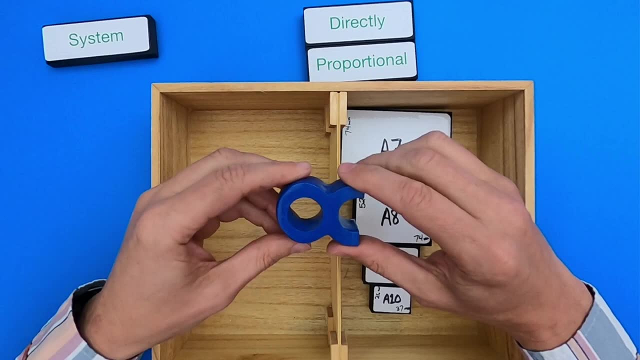 Now the symbol or the block that represents proportion is this block, and it's a weird symbol that you've never seen before. I think of it like an equal sign that you've kind of twisted off on the end, And I'll show you how to use that as we look for these proportional 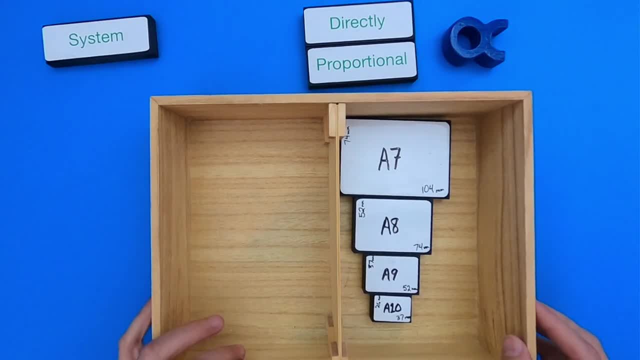 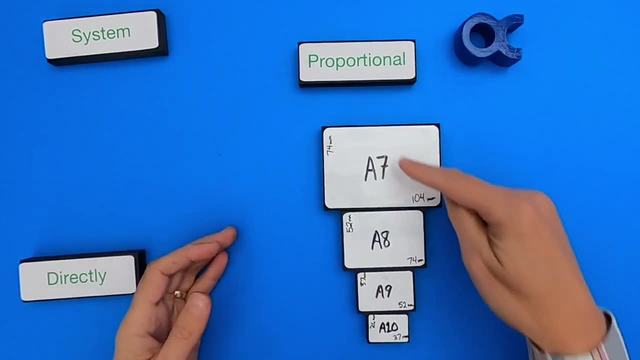 relationships. First thing, let me get these blocks out and then we'll take a look for those proportions. Now you can see on here that I have quite a bit of data. I've got the names of the blocks. I also have the length of the block in millimeters and then the width. 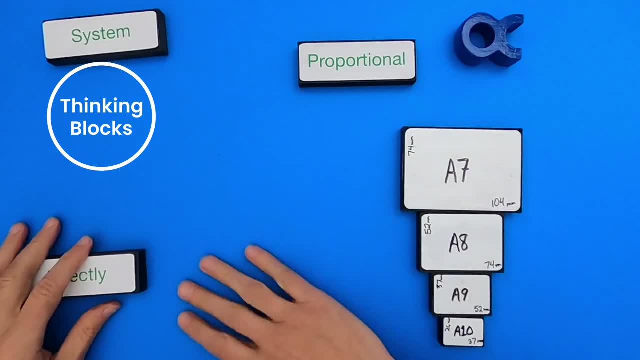 of the block, And so I'm going to do that. So here's my block And then I'm going to. So what I'm going to do is set up just a data table where I put all the data out so we can start to see it and looking for those proportionalities. 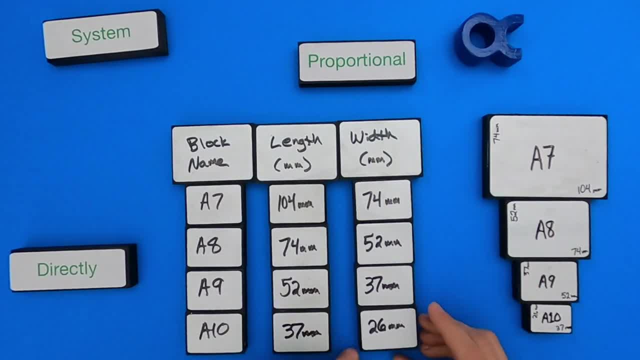 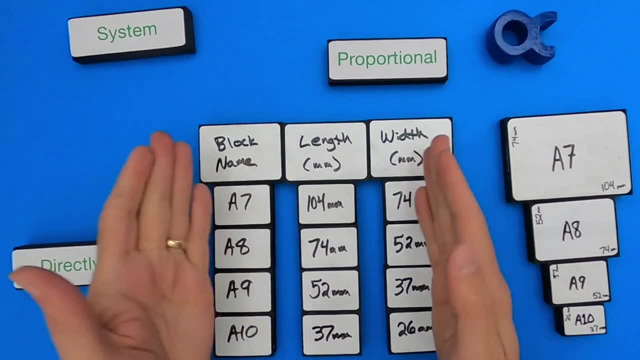 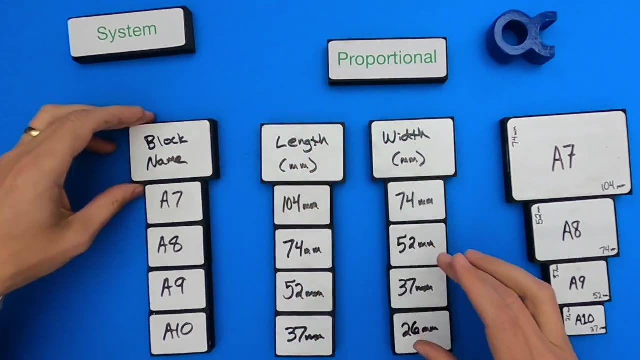 Okay, now that we've got the data, what we're going to do is start looking for proportional relationships between data sets, And what does that mean? So let me get these block names off to the side for a second, So if I move that over here. So what we're really looking for: 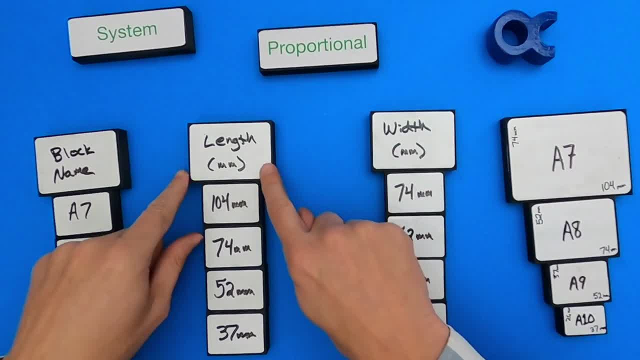 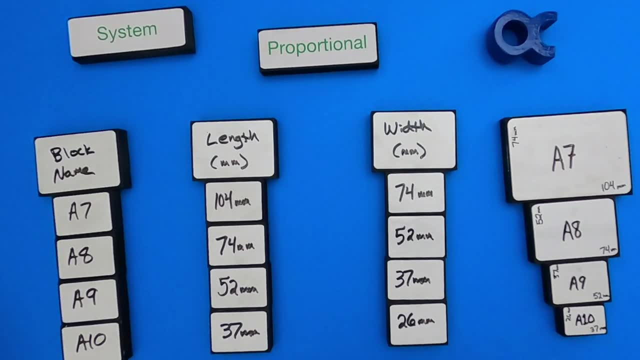 is there a proportional relationship between the length and the width? So the first way to start looking for that is number one. we could say: are they equal? so that's always before we get to proportional, we could say: are the two values equal? in other words, 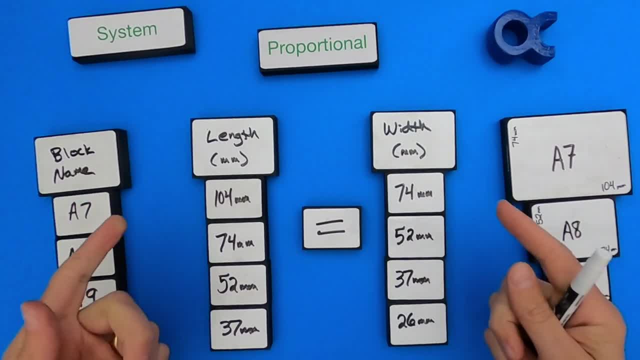 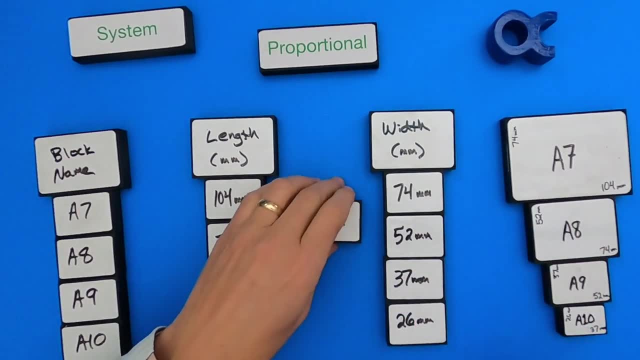 does 104 equal 74? i would say no. is 74 equal 52? i would say no again. so we would say these two data sets are not equal. but are they proportional? so if i draw that symbol again in the middle, so if we say, is there a proportionality between the left and the right, we're not just looking at 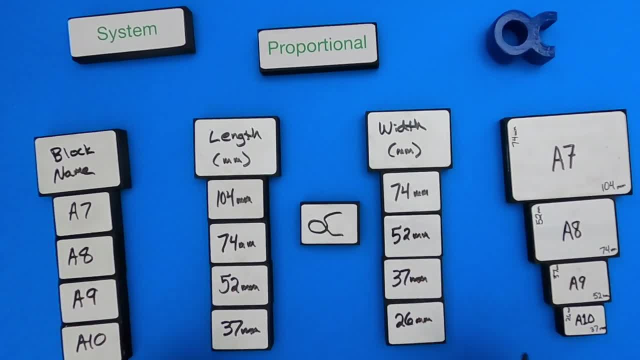 one or specific values. we're looking at the whole data sets and so a quick way to do that is: as this one goes down, does this one go down? i would say yeah, so that's a good sign that it's a proportional um, if another way to start looking for it is if this one is cut in half, so 104 down. 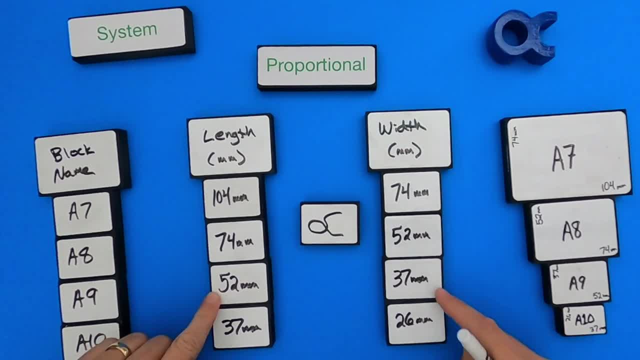 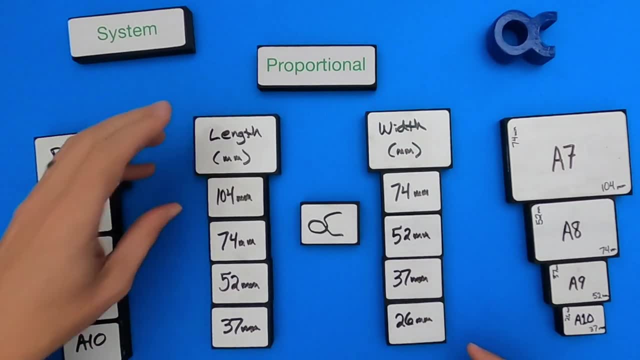 to 52. does this one also get cut in half? 74 to 37. or if i cut 74 and a half to 37, does this also go down the same amount and i would say, yeah, it also is cut in half. or if i triple this, do i triple that and so 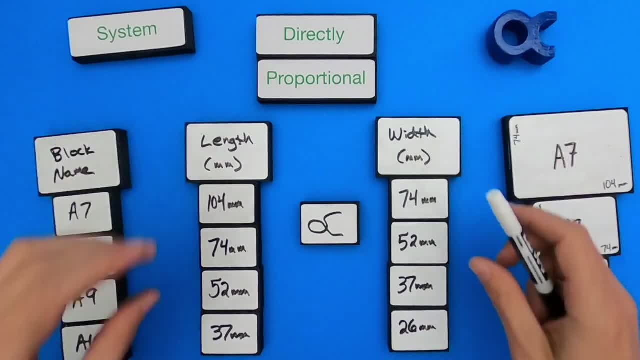 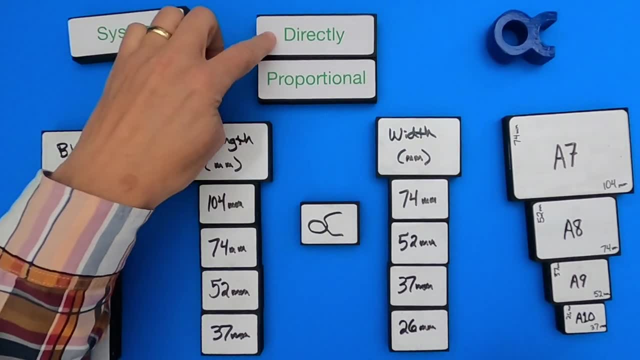 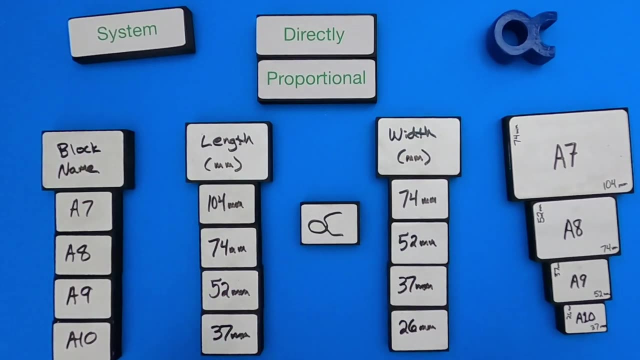 since it is, we would say that these two data sets are direct, directly proportional. another way to say that is: sometimes we'll call that a linear proportionality. in other words, if we were to graph it as this goes up, this is going to go up in an equal amount. now if we get the numbers out. 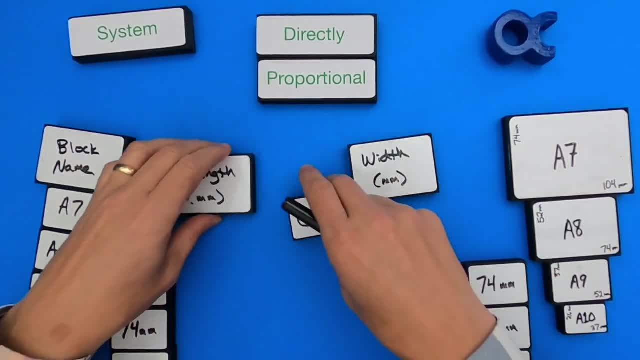 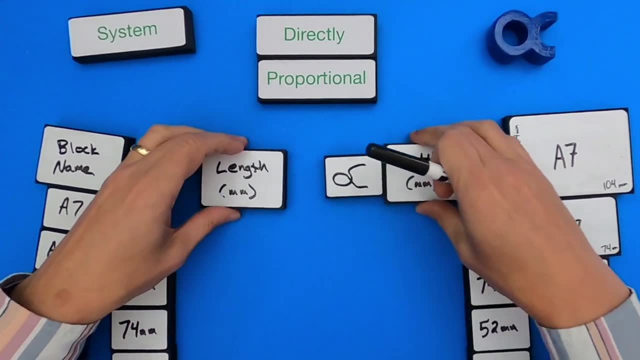 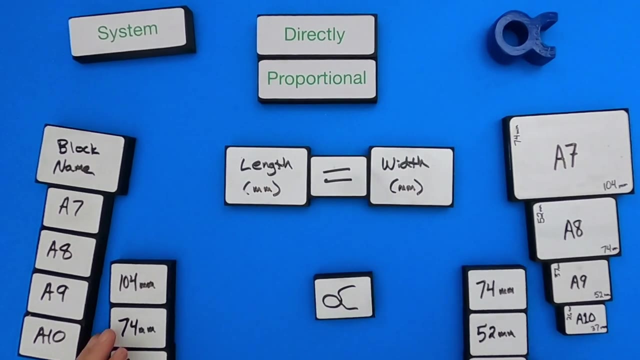 a second. so we could go like this: if we just get those out of the way, we could say that length is proportional to width. so we know that to be true. but i also could say: we know length does not equal width, but what could we do to those values so that we could make it equal? well, we 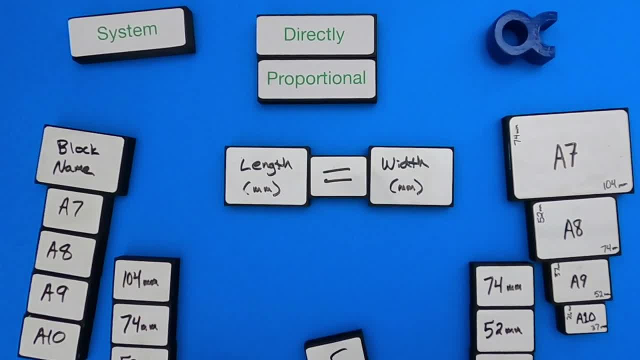 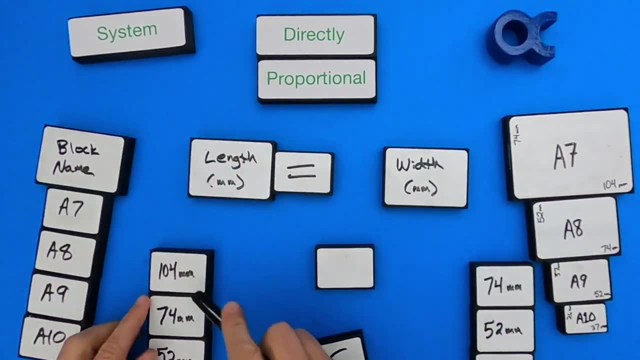 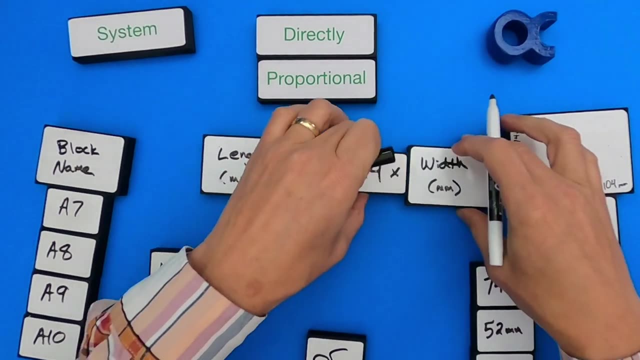 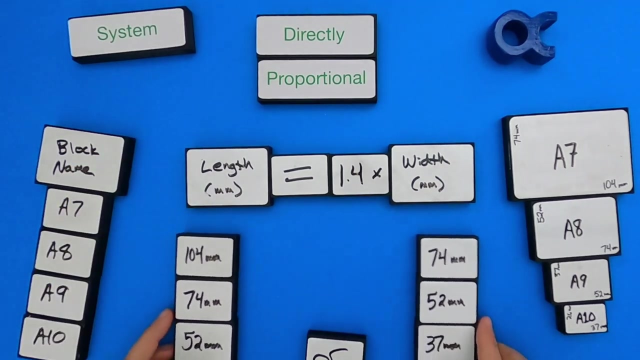 really need a constant. so we've got length and width. so if i have 104 and 74, a way to really figure this out is if i divide this by that, i could say the width times 1.4. so width, if we think of width as a variable, width times 1.4 equals the length. in other words, 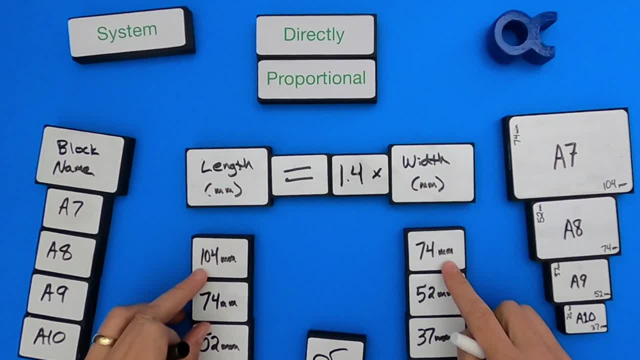 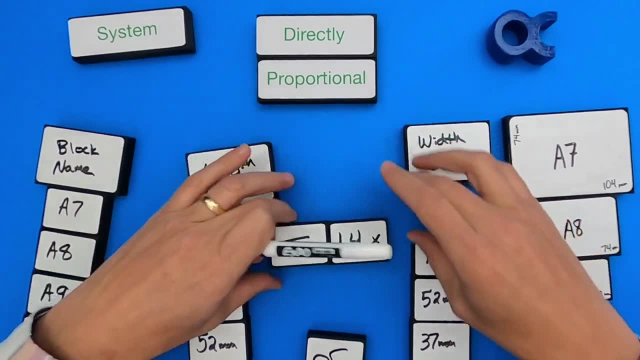 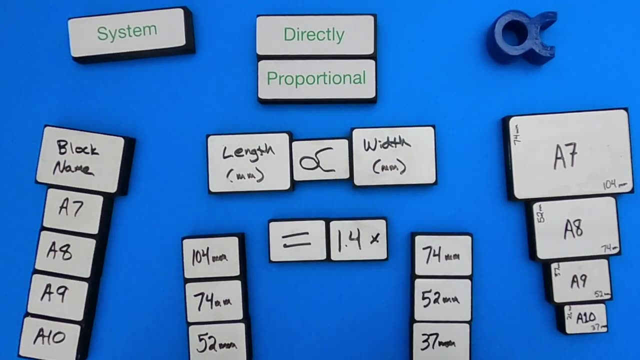 774 times 1.4 equals 104, and so you can see, like adding that constant allows us to say that those two values are going to be equal, and so that's the difference between being proportional and being equal, and you'll you get used to that sign because sometimes it will be a direct proportional. 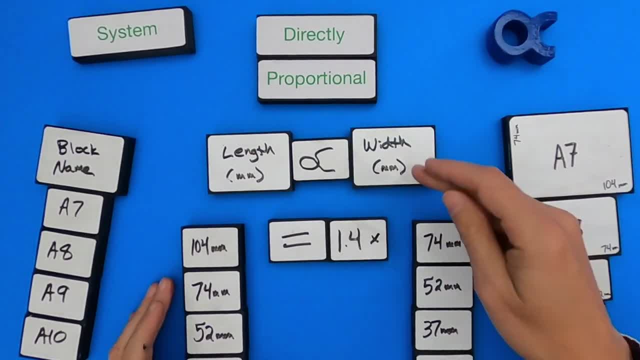 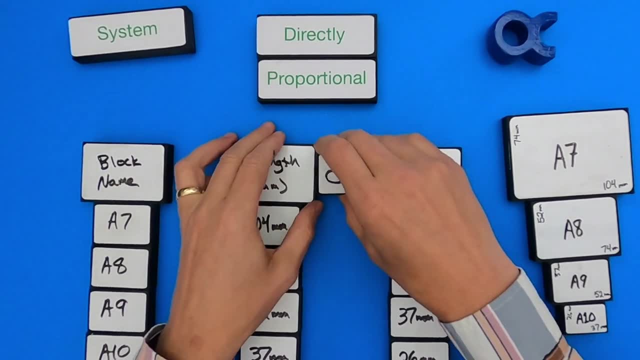 sometimes it will be a direct proportional, and sometimes it will be a direct proportional to the square of one of these values, and so if i get this out of the way for a second and put these back, we could also start looking at: well, let's look at the length and the block number, or maybe 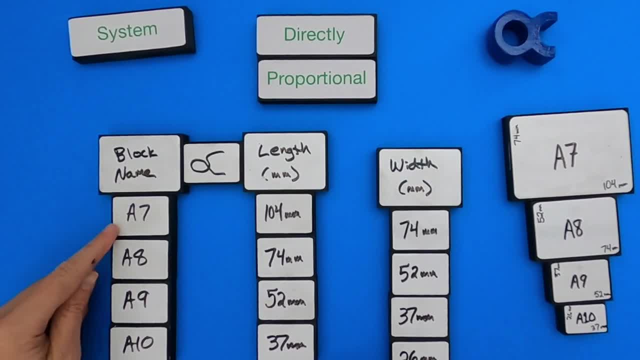 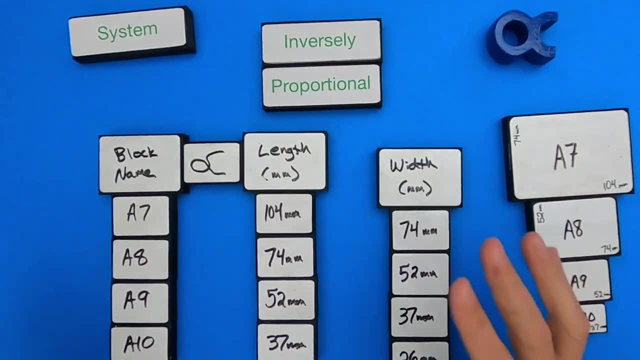 the block name. so as this goes down, can you see that the number is actually going up? so another thing in science that we have sometimes is called is it inversely proportional? and i'd have to do a little bit of math to figure out if this is inversely proportional. but that's kind of 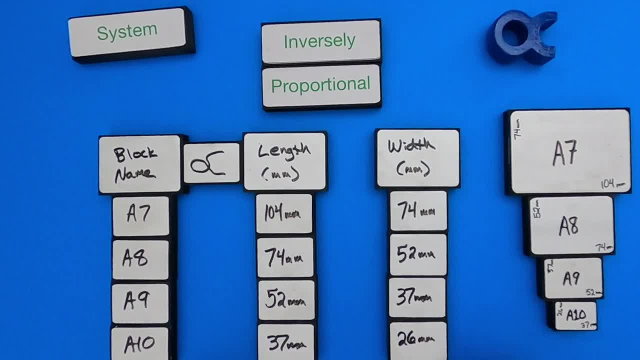 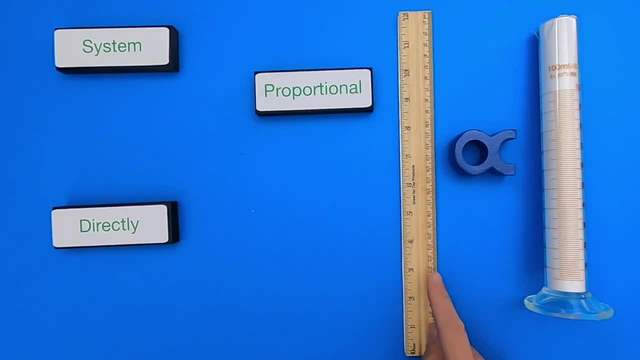 a way of comparing, especially the ratio between the change of these. so what i'm going to do is clean this up, and then i'll give one that you can try. okay, for the second example, we're going to look at the graduations in this ruler and the graduations that you see on the side of a graduated cylinder. 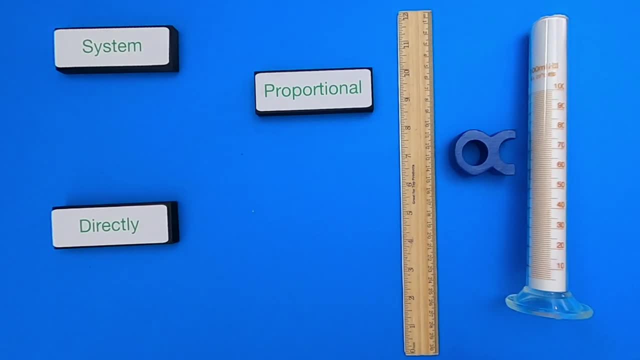 and we're going to see: is there a proportionality and if so, what is that proportionality? so the first thing you want to do is you want to set up the system, or define the system. so in this case, the system are going to be the cylinder, so the graduated cylinder- and the ruler, the graduation. 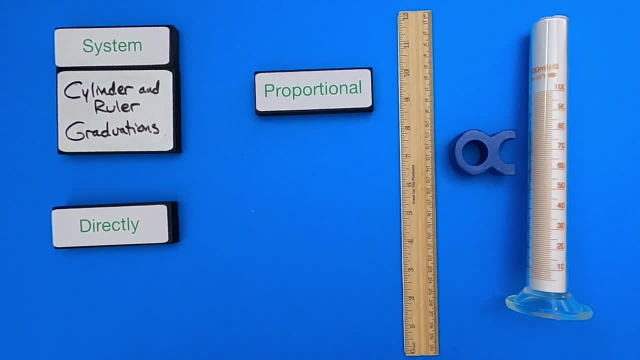 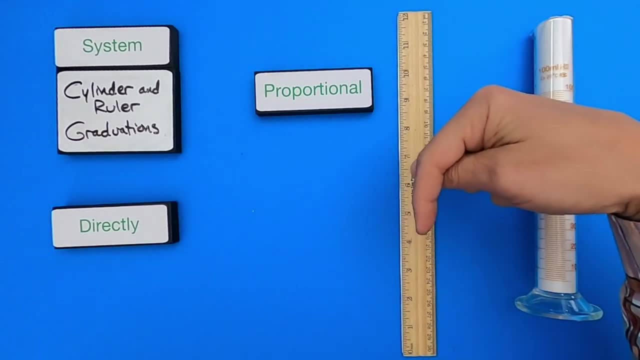 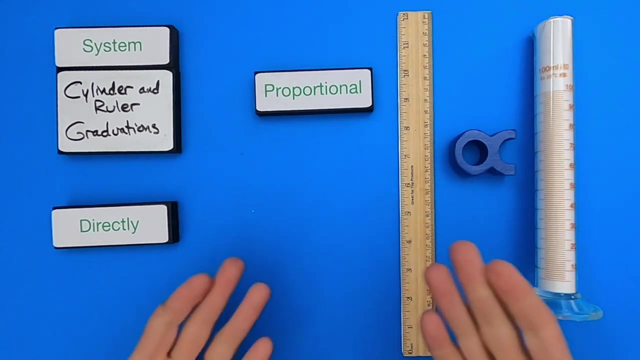 or the marks on the sides of those. so what i'd like to have you do is- i've included a photo of this, putting them right next to each other, and i'll include that in the thinking slides down below. so take a second to calculate or measure the data and then start looking for proportional relationships. 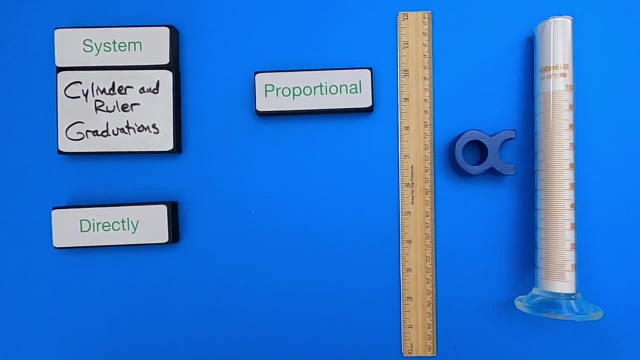 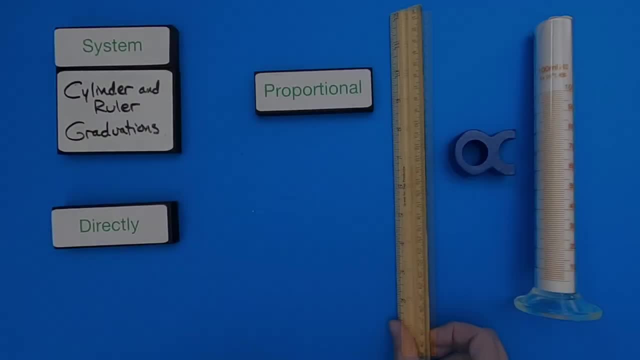 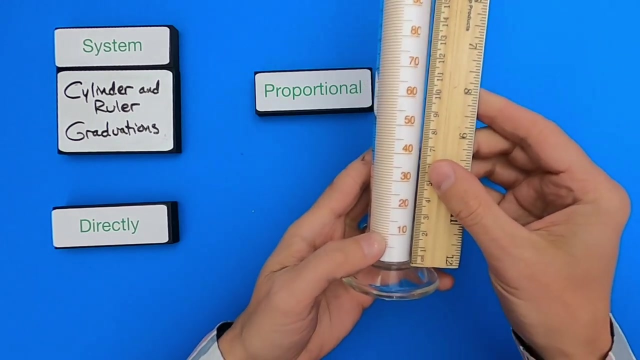 so pause the video, try to do that on your own and then come back and we'll work through this one together. okay, so what i would do is i would hold the ruler right up to the graduated cylinder and if i do that right, i can see that they are. i can see, at least see the relationship. in other words, when i hold 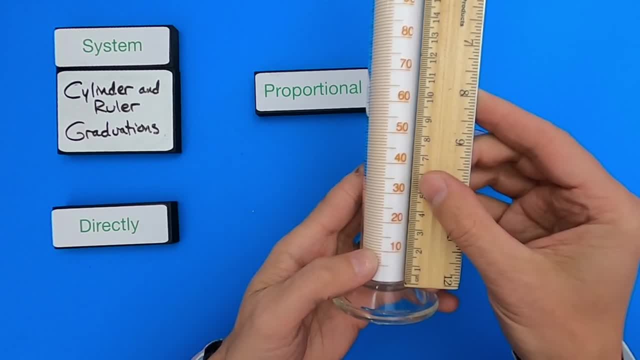 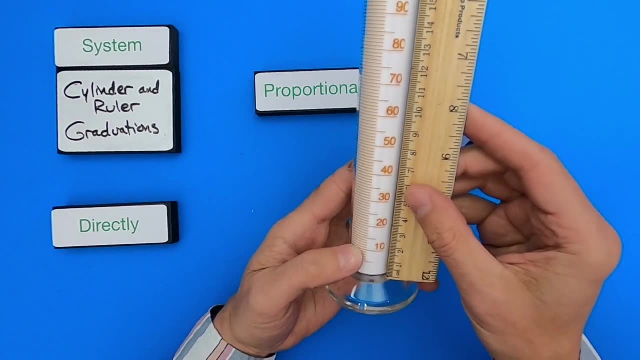 the uh ruler up to the graduated cylinder i can see that when it's 20 milliliters in the graduated cylinder it's 30 milliliters. so that means the graduated cylinder is 30 milliliters and the graduated cylinder is participate in that same process. 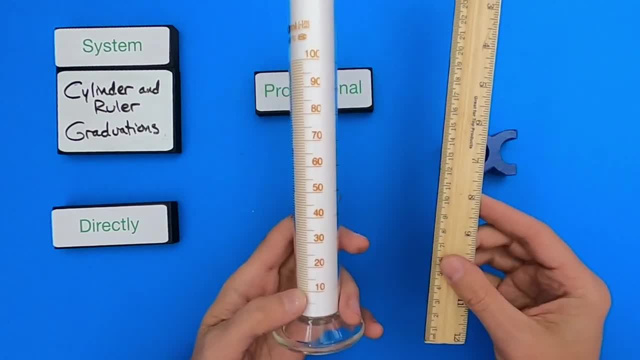 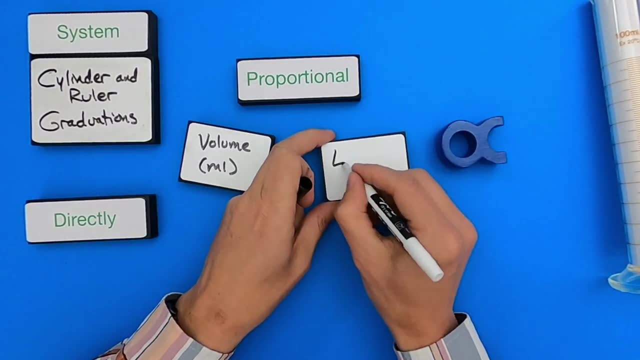 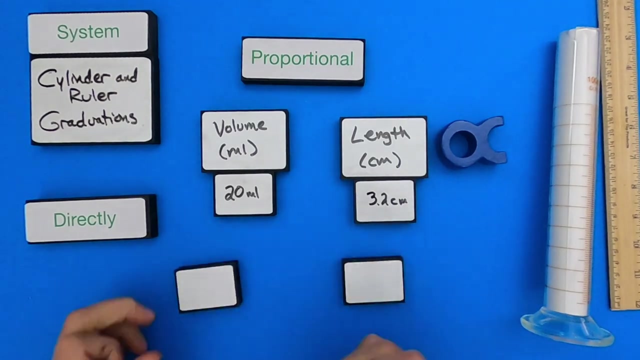 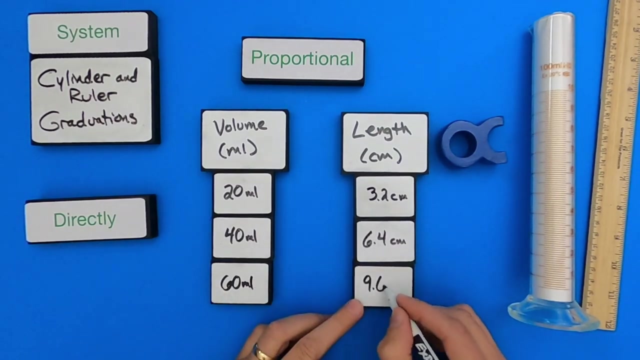 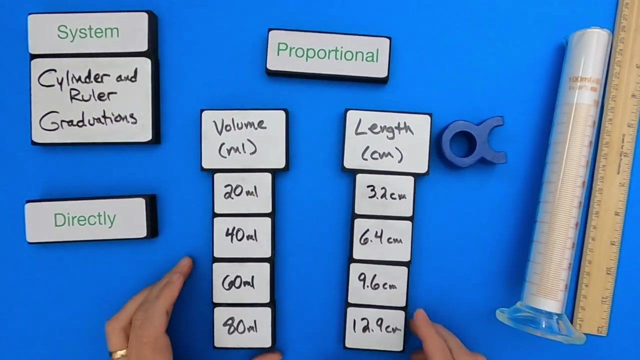 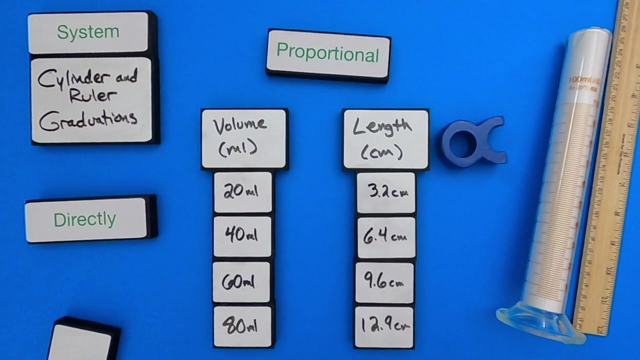 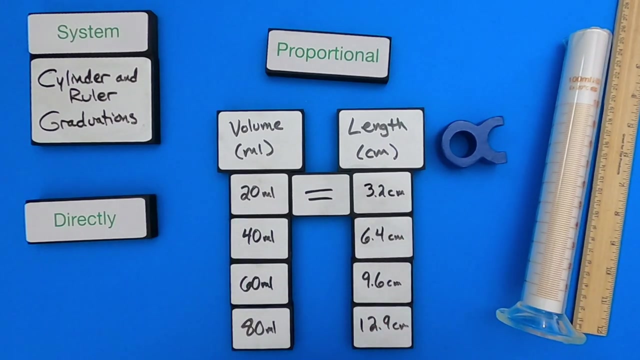 3.2 centimeters, And so what I'm going to do is take a second to gather the data, and then we'll look for proportionalities. Okay, the next step is to start looking at the two and comparing the two, And so the first thing I always do is to just say: well, are they equal? Are the two data sets equal? In other words, does 20 equal 3.2?? I'd say no. So I would definitely say it's not equal, but let's hold on to that. 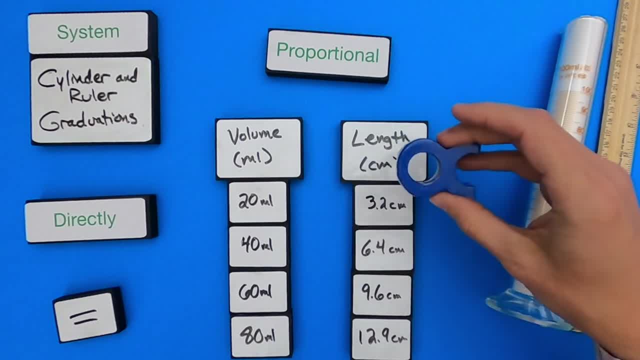 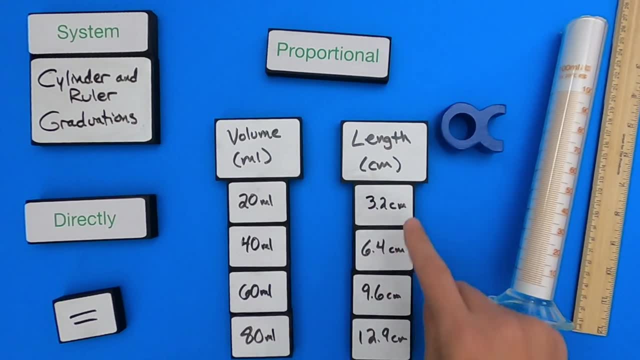 The next thing is where you start looking for proportionality, And so, again, a good way to see is the change in this one kind of matching the change in this one, And I would say, yeah, as this one goes up, this one's going up. A really good way to look at that is: as I double this, so 20 to 40, does this double? Yeah, If I triple this. so this is 20,, now it's 60, does this triple? Yeah, exactly triples. 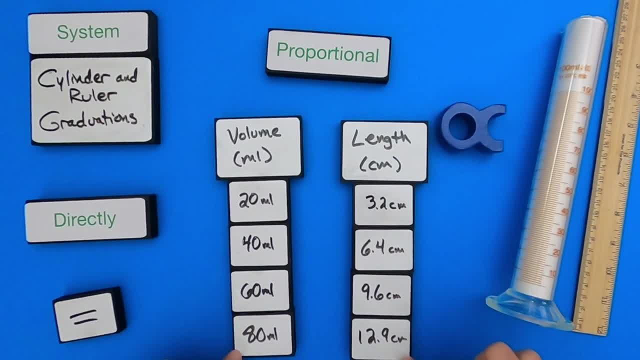 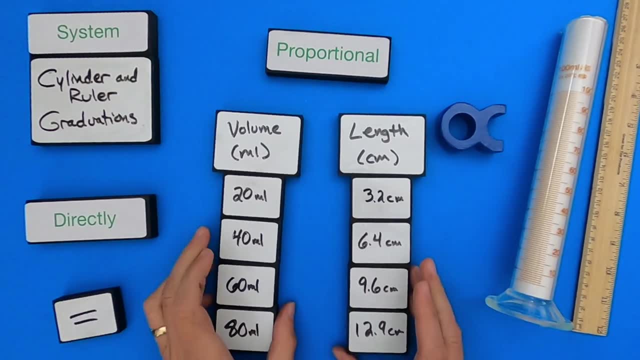 Or if I quadruple this, or if I take this 60, or let's say 80, and I take that in half, is half of that equal to half of that? And it's not exactly, but it's pretty darn close. And so what I could say is that these are proportional. 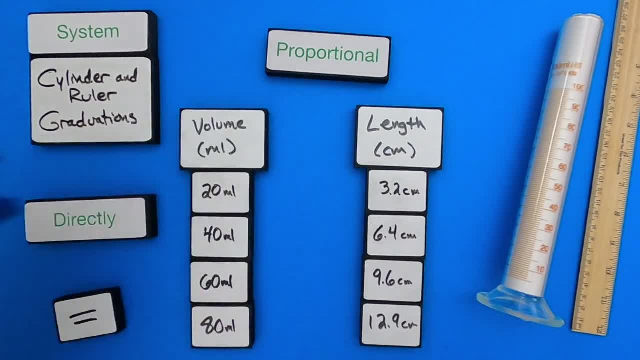 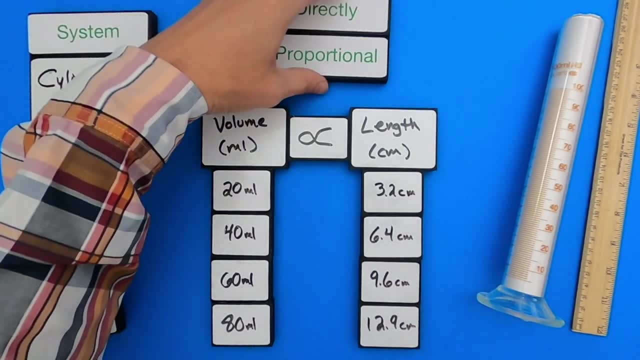 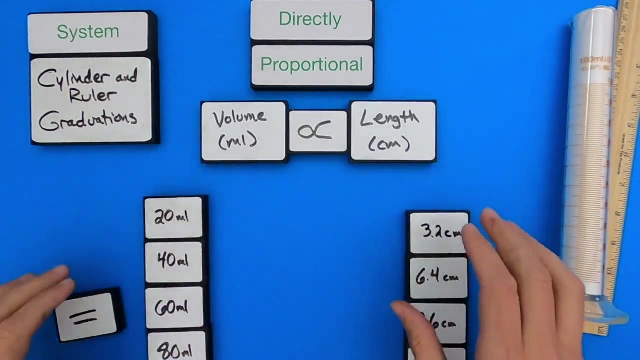 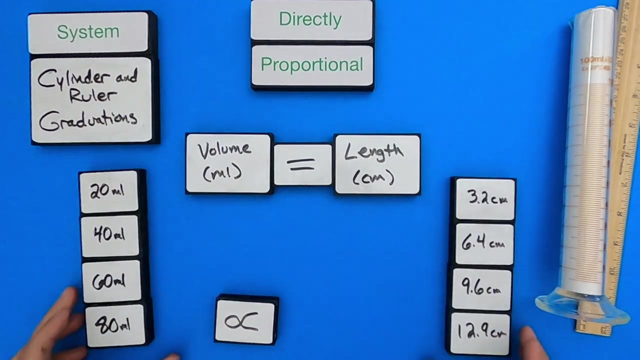 In other words, volume is proportional to length, Or, if I write it out, there's a proportionality and I could say that there is a direct proportionality between the two. If I start to calculate that, remember. so if I take these off, we can't say that volume equals length. So that's not true. 20 does not equal 3.2. 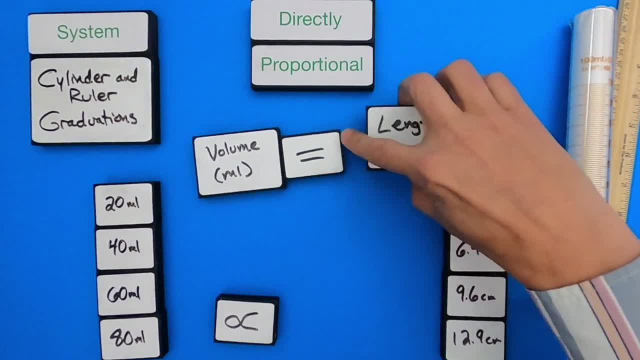 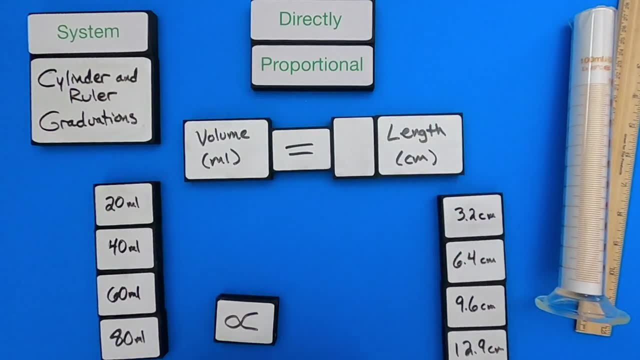 But for me to make it equal have to multiply it. times, sum Lots of times. in science we'll call that a constant. So we could say: let's multiply that times a k. we could say So a k value which is just stands for a constant. 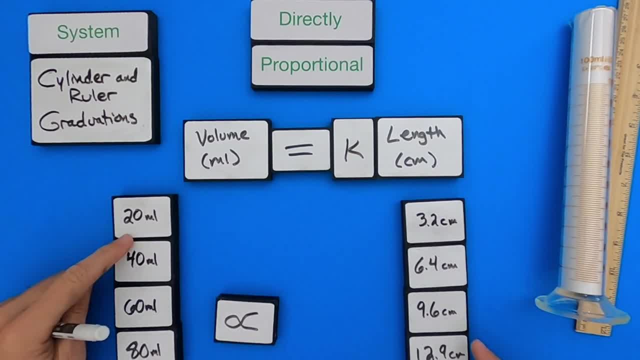 value And I think we could figure out what that is. So if this is 20, then this is 3.2, and this is 20 and this is 6.4.. So it's going to be that ratio between the two which I might have to use. 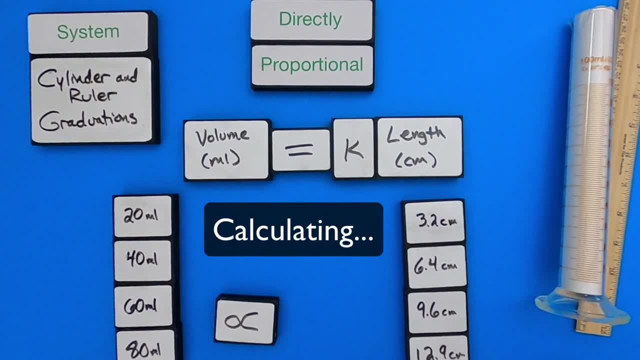 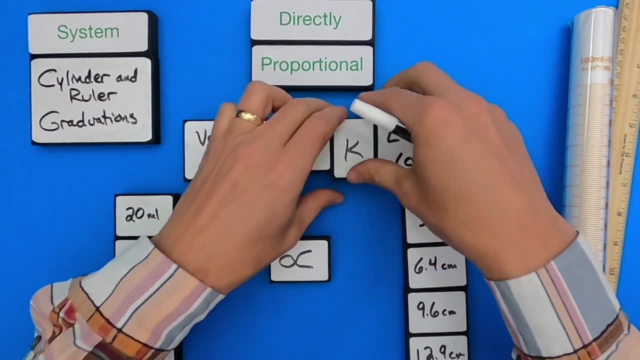 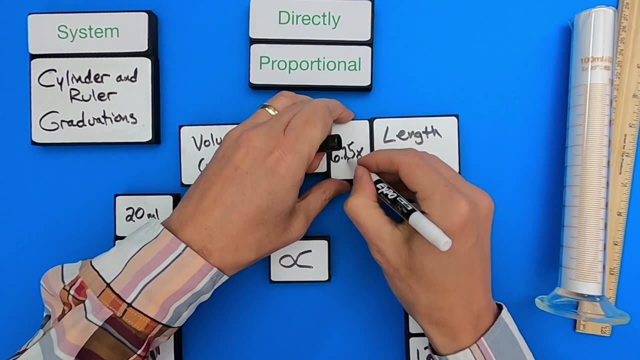 a calculator to do So, the value that I'm getting is 6.25.. In other words, if I take 3.2 times 6.25, so we could say the length times a constant of 6.25, then the length times 6.25 equals the volume. 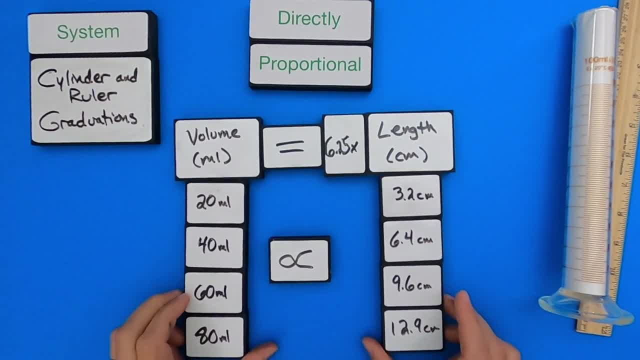 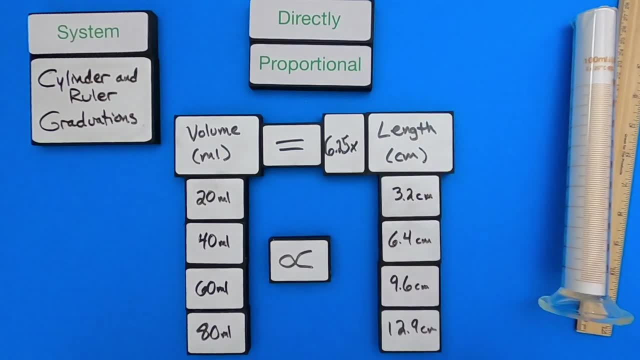 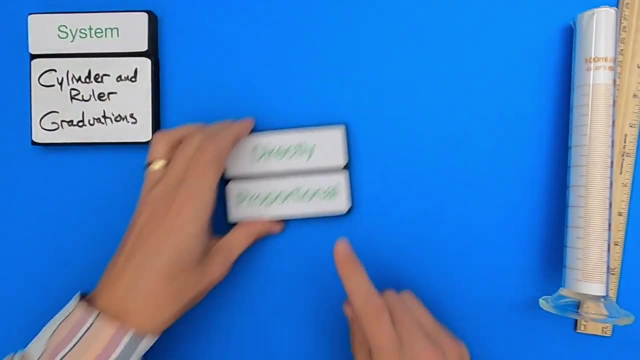 And so hopefully you see the value in looking for proportionality- it allows us to find what is the equivalent. So what I've done is I've put some examples down below in the thinking slides and you could take a look at those. I hope, as we do this, that you're not getting this idea that everything is. 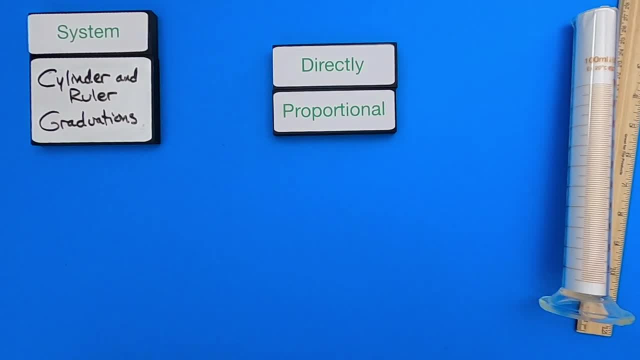 proportional, or everything is directly proportional. So I asked my wife to just make up some data, and so she gave me some data. The data is 7,, 4,, 6, and 8. And then I just wrote some data as well. 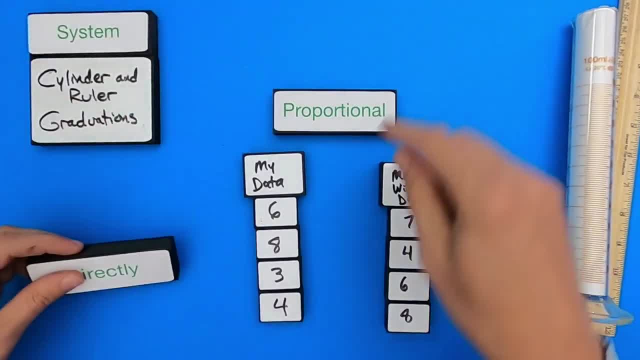 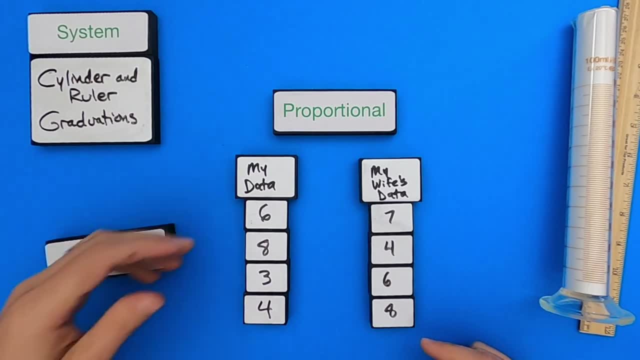 So my data is 6,, 8,, 3, and 4.. And so as I look at this data, you can see it's random. We just thought it up. But I could start looking for proportional. Is it proportional? I would say?